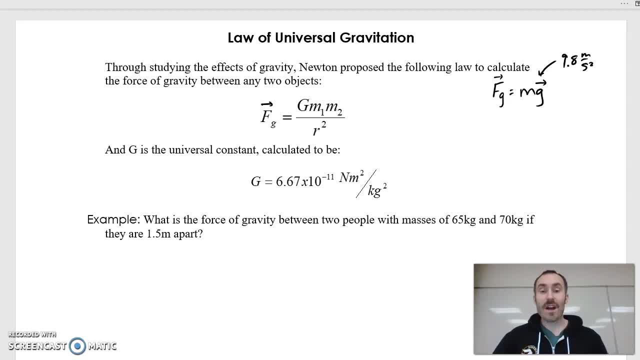 is that we can figure out the force of gravity between any two objects whose masses are known and the distance between them is known. So this g here is the universal gravitational constant, And so you can see right below, that is 6.67 times 10 to the negative 11 Newton meters. 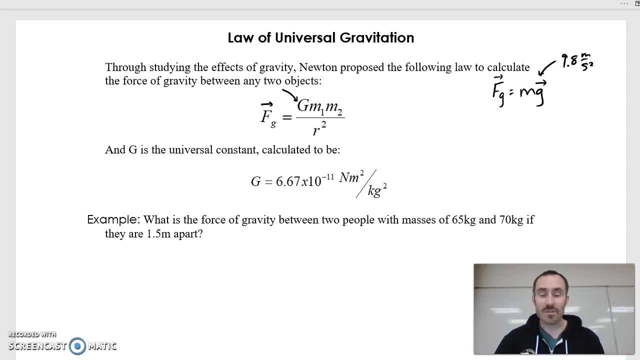 squared per kilogram squared, The crazy unit. but it's important to make all the other units work out in the question. Okay, so you don't need to worry about that unit. Very important for our actual calculations. These other two things, m1 and m2, these are the 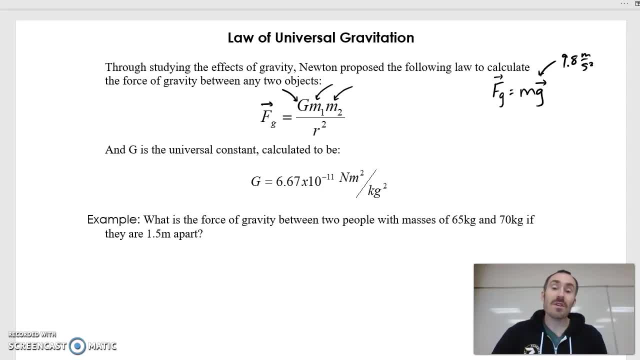 two objects' masses that you're talking about. Okay, so maybe it's you and the Earth. So then you would put in your mass in kilograms and the Earth's mass in kilograms. Maybe we're talking about the Earth and the Moon, Or the Sun and the Earth, or something like that, And then this r value over here. this. 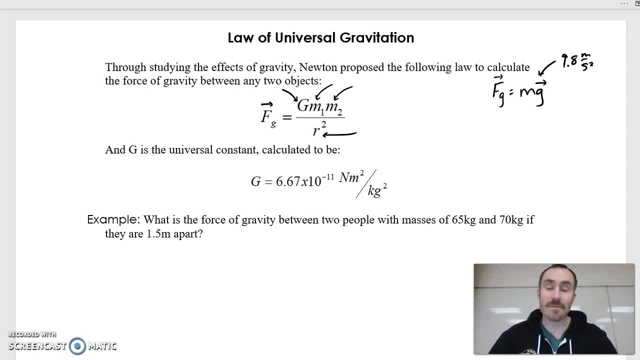 is important. This is the distance between planetary centers again. So it's the same thing as the k equals r cubed over t squared, That r value is the distance between planetary centers, Or in this r values case, it doesn't have to be planetary centers, You could figure. 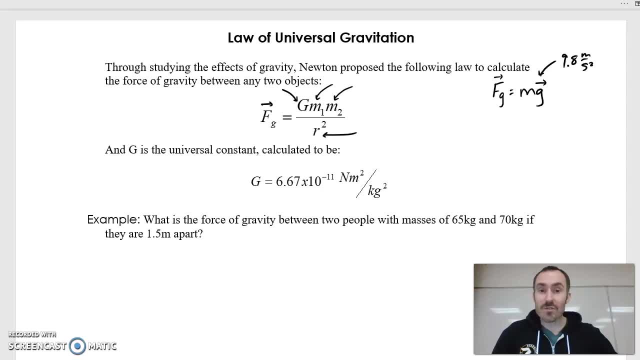 out the force of gravity between you and the person who's sitting there, And then you would be left with only one person sitting beside you. That also works. You just need to know the distance between your center and that person's center. So when we're calculating, 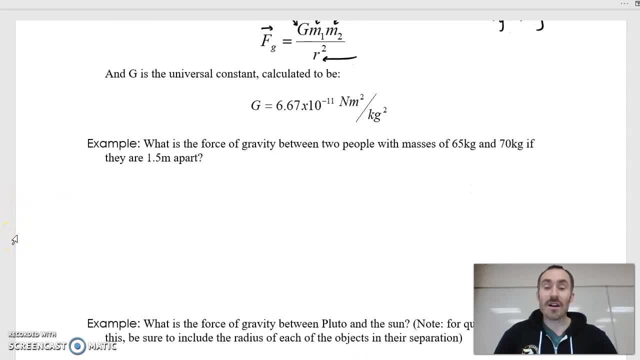 the force of gravity between two people, then it's not a big deal to go from center to center, because the difference between going from my center and going from my shoulder is very little. That distance is only what? 1? 1?. 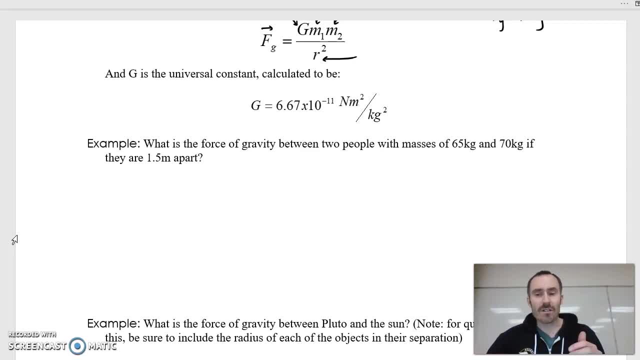 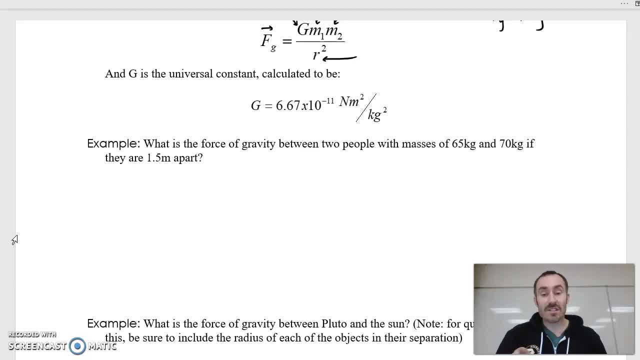 objects, it's important that you take into account the distance from the center of the object to the edge of the object in your calculation, in that r value. So let's start with a simple one and then we'll jump to a bit of a more complicated one. What is the force of gravity between two people? 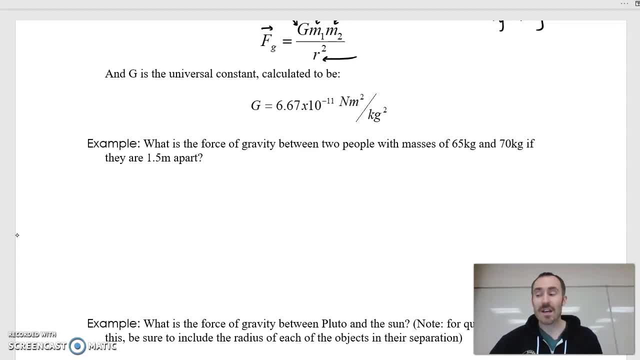 with masses of 65 kilograms and 70 kilograms if they are 1.5 meters apart. We're assuming that that's 1.5 meters from center to center, But again there's not much difference between center to center and outside shoulder to outside shoulder. So the force of gravity between them. 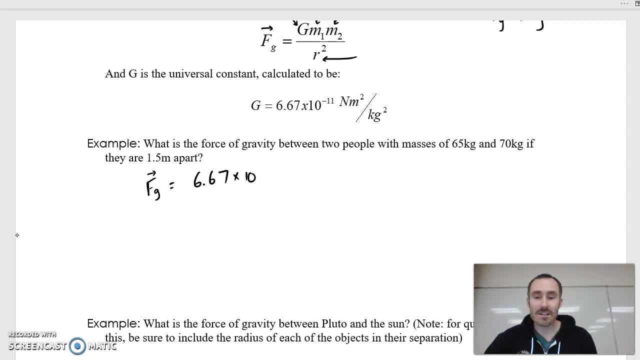 is 6.67 times 10 to the negative 11 crazy unit times 65 kilograms times 70 kilograms. And all of that is divided by the r squared, which is 1.5 squared, And so the force of gravity between those two people is 1.34 times 10. to the negative seven newtons, a very, very 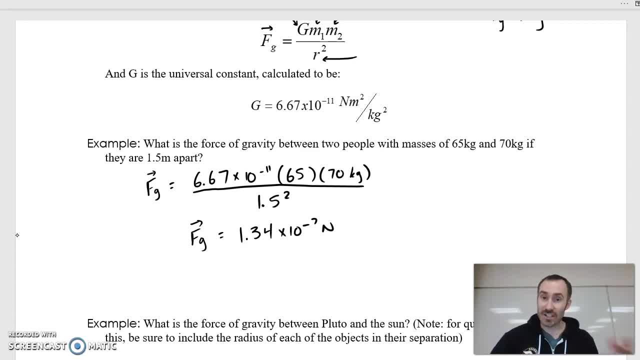 tiny amount, which is why you don't feel gravitationally attracted to the person beside you who's 1.5 meters away, And so the force of gravity between those two people is 1.34 times 10 to the negative seven newtons- a very, very tiny amount, which is why you don't feel gravitationally. 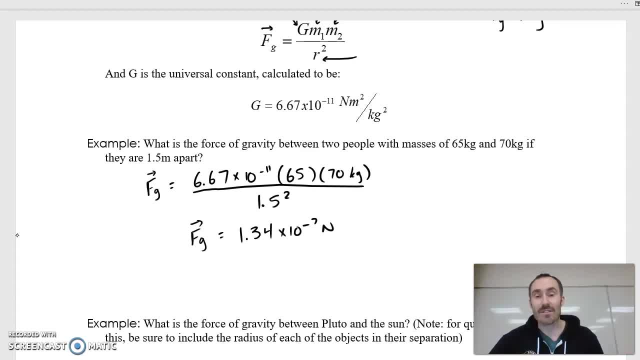 attracted to the person beside you who's 1.35 meters away. It's just such a tiny, tiny amount of gravity. So in order to increase that gravity, you've got to increase those masses by such an enormous amount, And so in the second example we're going to see that happening. What is the? 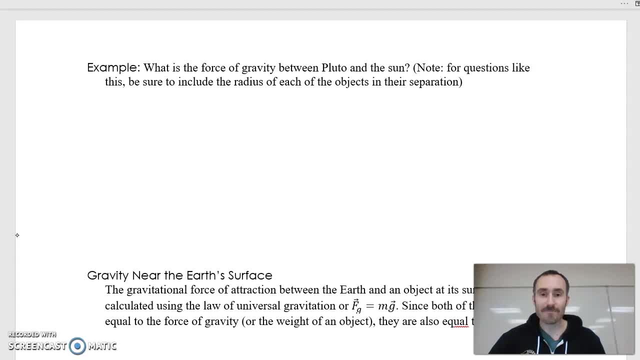 force of gravity between Pluto and the sun. It tells us nothing else. It doesn't tell us the force of it, doesn't tell us Pluto's mass, the sun's mass, the distance between them, nothing like that. But if you look at the force of gravity between Pluto and the sun, you'll see that the 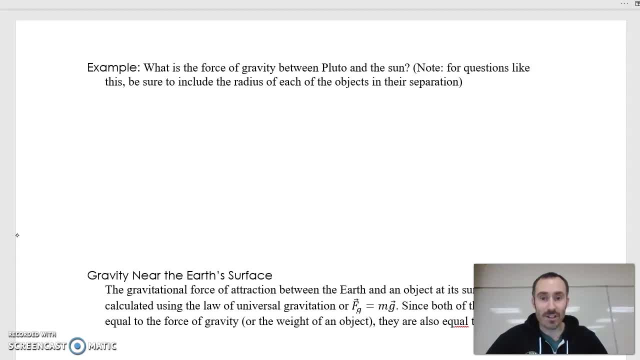 force of gravity between Pluto and the sun is equal to the force of gravity between Pluto and the sun, And so, if you are following along in this course, on the back side of your formula sheet you will see a table that has all of that information in it, And so we then can use the force of gravity. 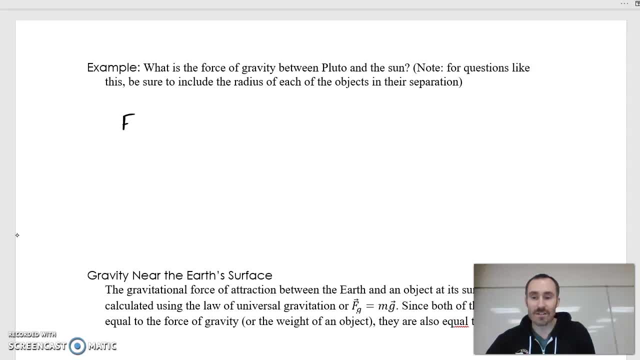 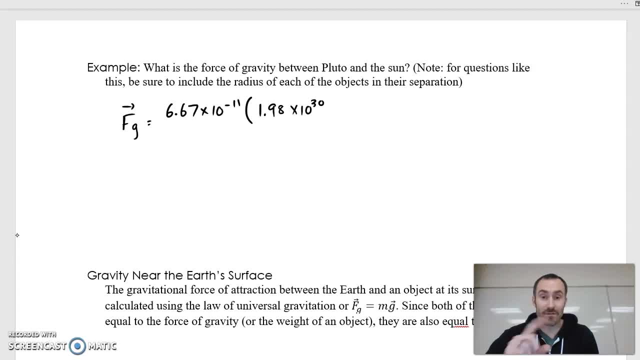 times 10 to the negative. 11 times the mass of the sun, which is 1.98 times 10 to the 30 kilograms. You can find that on your formula sheet. times the mass of Pluto, which is 6 times 10 to. 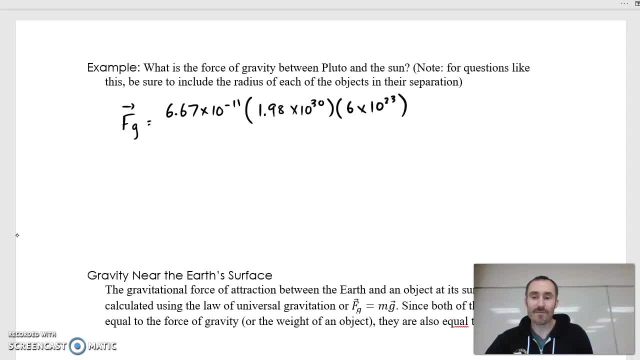 the 23. And we'll divide that by the distance between the center of the Sun and the center of Pluto. Okay, so we're going to put in Pluto's radius of orbit here 5.9 times 10 to the 12. That may have been updated on your formula sheet. I can't quite. 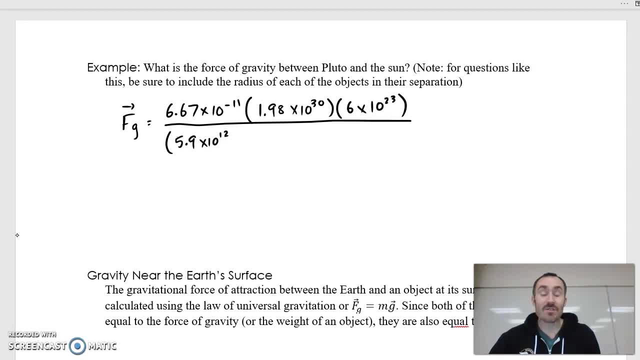 remember, but we're going to go with this for now. So that's the radius of orbit, That's from the surface of the sun to the surface of Pluto And so onto that we need to add the radius of the sun and the radius of Pluto, Because when we look at our, when we look at the radius of orbit, 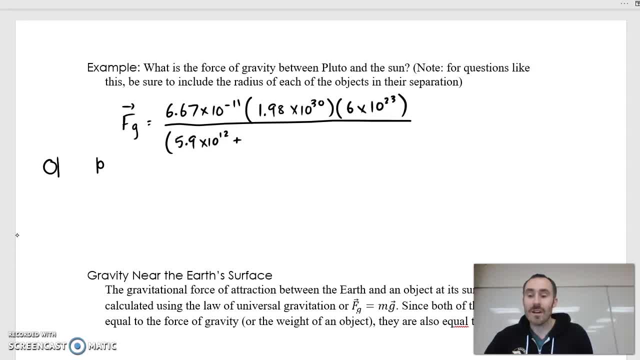 it's from here to here. So we need to also include this distance here. And we need to include this distance here Because we need the distance from center to center, So we get the radius of Pluto's orbit, which is this piece, And then we also have to add this piece here and this piece over here. 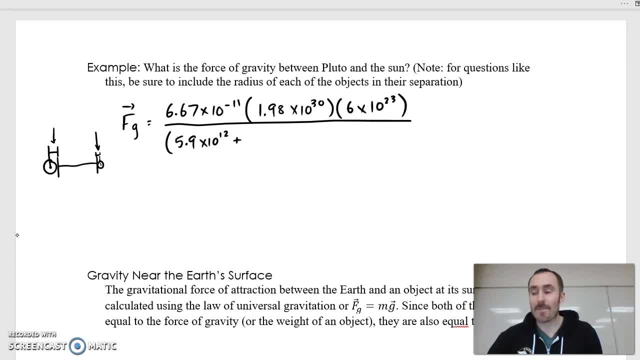 And we can get those from the radius of each planet. Okay, And so the radius of the sun is 6.95 times 10 to the 8. And the radius of Pluto is 3 times 10 to the 6.. That's all in meters, And this whole thing is the center to center distance, And that's. 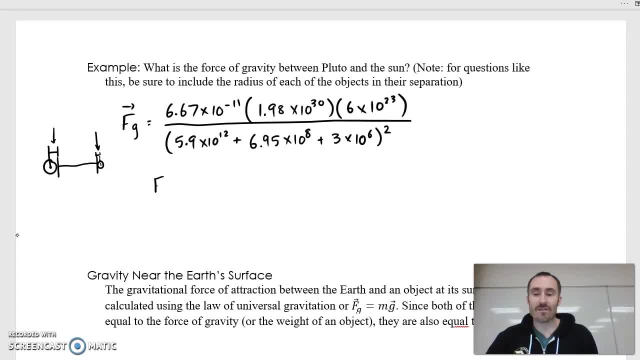 squared. Okay, And so then we can figure out: the force of gravity is equal to 2.28 times 10, to the 18 Newtons, Far, far bigger than the force of gravity between those two people. Okay, So this is not a particularly difficult question to do either, But you do have to. 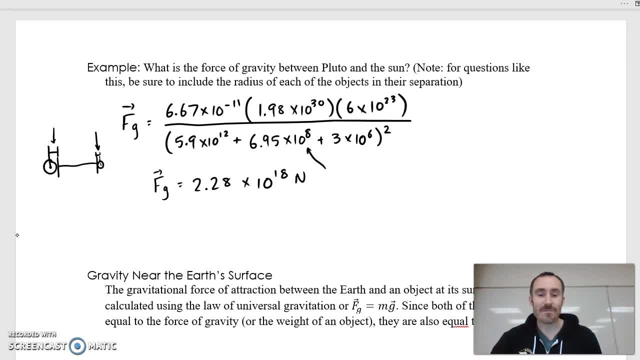 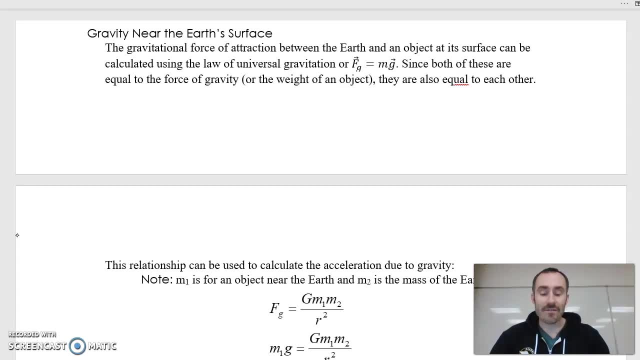 remember to put in the radius of each planet when you're calculating that r value from center to center. Now we're not saying that that Fg equals mg formula. this one, we're not saying that it was, It wasn't wrong. it's correct in just certain circumstances, which is why universal gravitation. 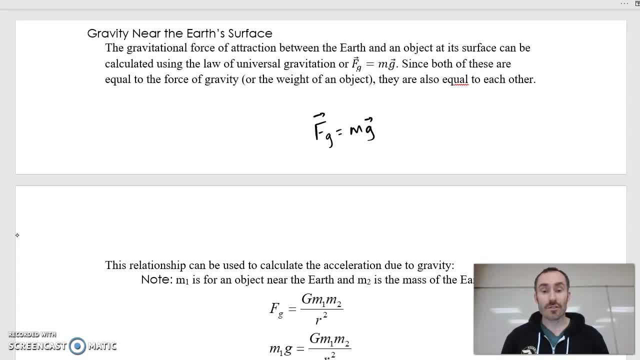 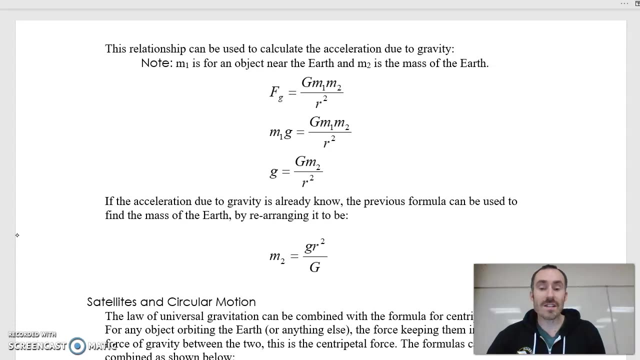 is a better formula than this one, because it applies to all circumstances. It's universal, But we can set them equal to each other in certain circumstances, and that yields some important results. Take a look at this. So if we say that the force of gravity is the universal gravitation, 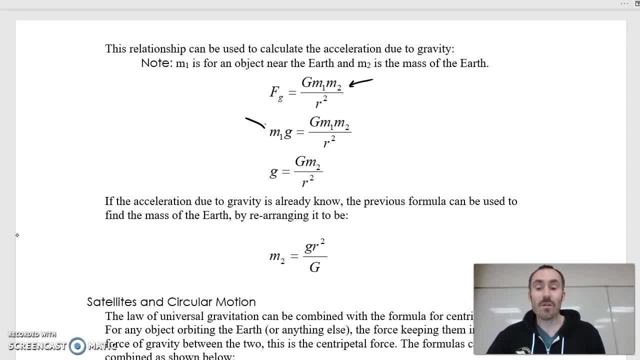 formula right over there, And then we also put in the near-Earth formula We can divide by m1, so that just ends up cancelling this guy out- in order to get a formula for the acceleration of gravity near the surface of any planet. 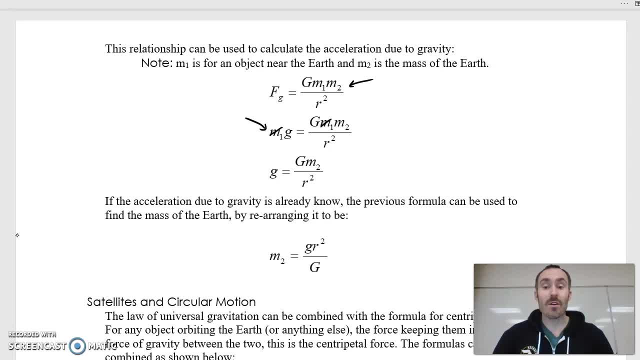 Okay, so at this point we're not necessarily talking about Earth, but any planet would do this, well. Well, so if you know the mass of the planet itself, then you can figure out the acceleration of gravity on that planet. And you need to know the radius of the planet, right? 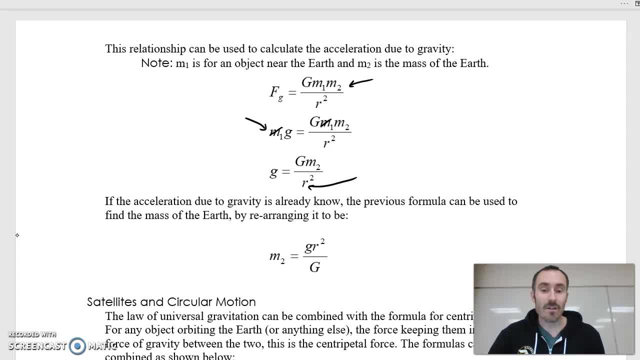 So this r-value over here, or whichever r-value you want to use over there, is the distance from the center of the planet to the surface of the planet. right, Because you're imagining yourself standing on the surface of the planet, If you jump a little bit. 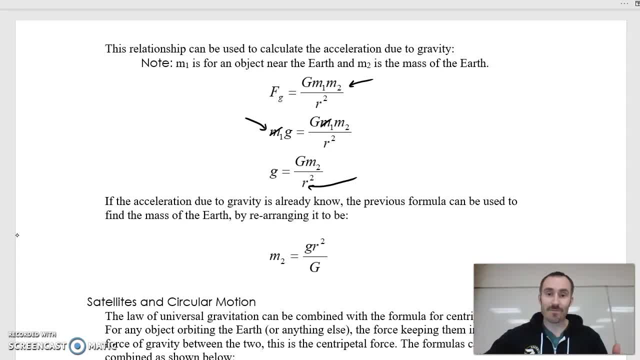 what's your acceleration when you're falling back down? Well, what's your acceleration on the way up as well, I guess? Right, it would just be the opposite way, because it's slowing you down. But this is the radius of the planet. 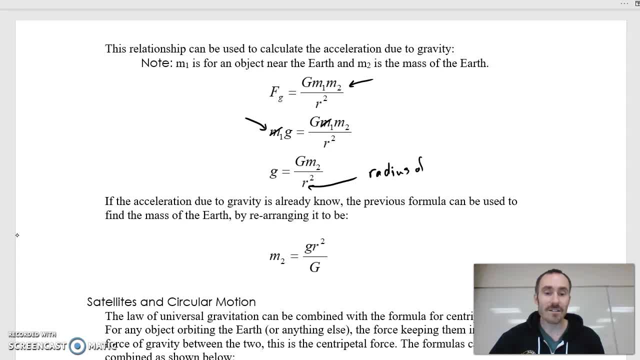 So if you know the radius of the planet and you know the mass of the planet, you can figure out the acceleration of gravity on that planet. Now I should point out that it's not always written like this: gm1m2 over r-squared. 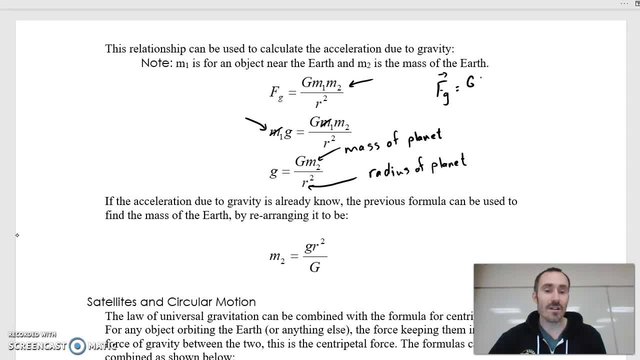 Sometimes it's written like this: g big M, little m over r-squared, And this big M over here, this is the mass of the planet. Okay, And then when you split this force of gravity into its, you get mg equals g big M, little m over r-squared. 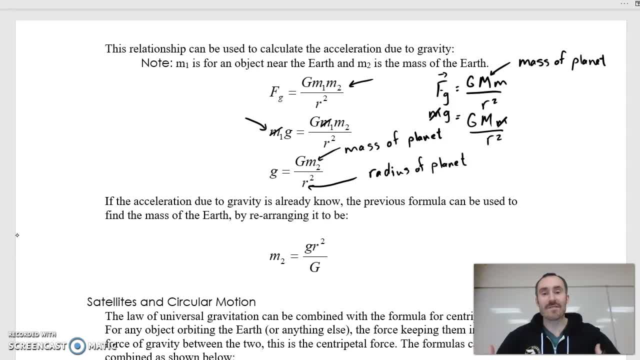 and it's the little m's that cancel out. It's the mass of the person who's jumping. if that's still the example we're going with, Okay, so it works the same way. It's just that that big M that you might see in the formula. 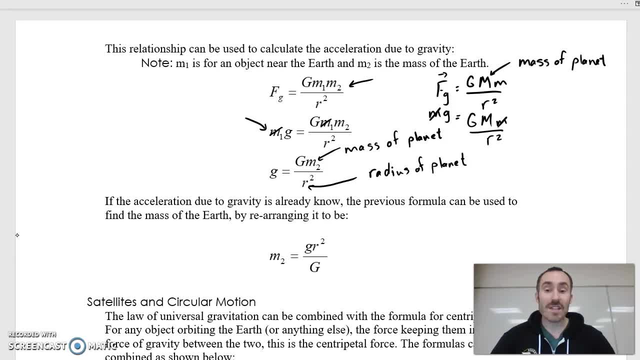 is the mass of the planet. Now, if you're standing on that planet and you can experiment to figure out the acceleration of gravity on the planet, then you can see that the mass of the planet is the mass of the planet. Okay, 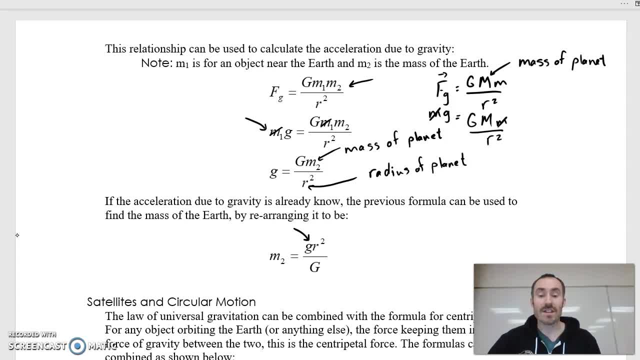 You can use this version of the formula. you can put the acceleration of gravity you've just found in there and you can use the radius of the planet, which can be calculated using astronomy measurement tools, and you can then calculate the mass of the planet. 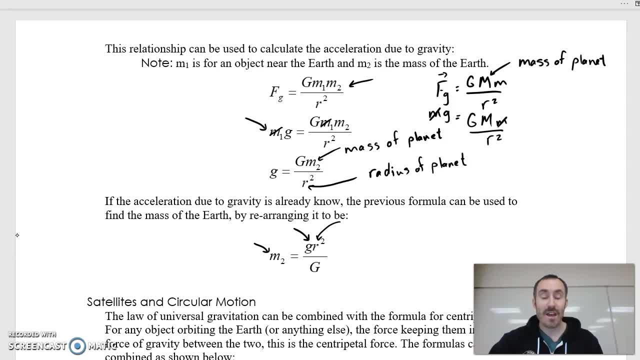 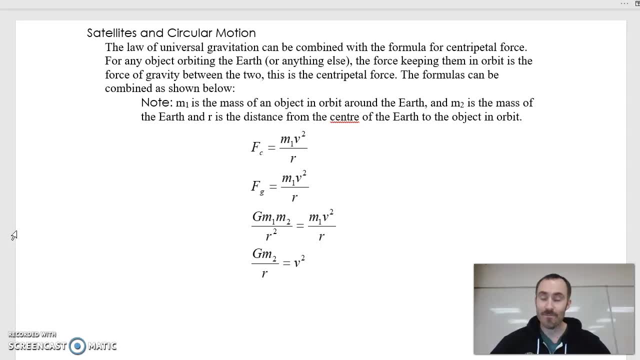 Okay, so that's just another way that you could possibly use it. And finally, the third way that you can use universal gravitation is with circular motion, is with satellites zooming around the Earth. okay, And so the force of gravity is the thing, is the force that's causing satellites to 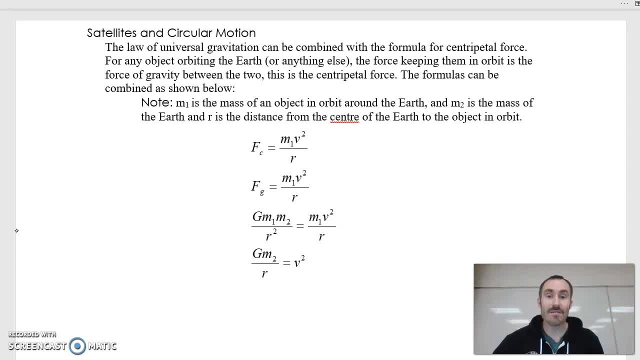 continue to revolve around the Earth, right? If gravity suddenly stopped existing, then the satellite would just zoom off into space tangentially. Okay, and so it's gravity, the force of universal gravitation, that's continuing to make that satellite move in a circle. 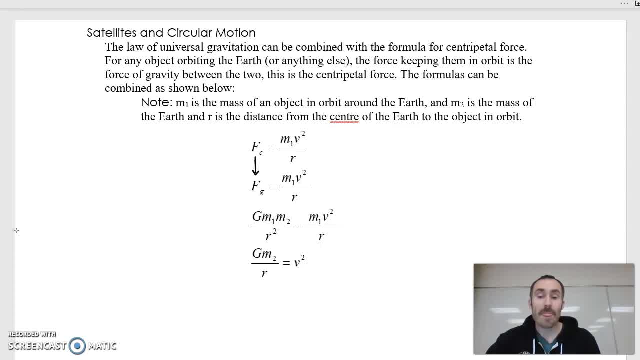 And so that's what's happening here. We can take the centripetal force and call it what it is: the force of gravity, and that gives us mv squared over r. This m1 is the mass of the satellite satellite, And a satellite does not have to be a man-made satellite. that's immediately what comes to. 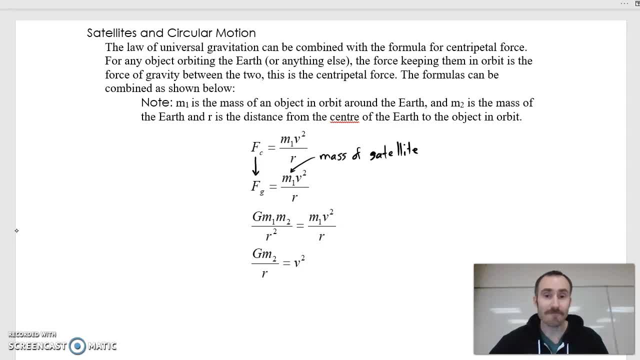 my mind. But the Moon is a satellite of the Earth, Earth is a satellite of the Sun. anything that revolves around something else is a satellite of that thing, And so this would also work for figuring out the velocity of the Moon. So we can replace Fg, the force of gravity, with the universal gravitation formula, and